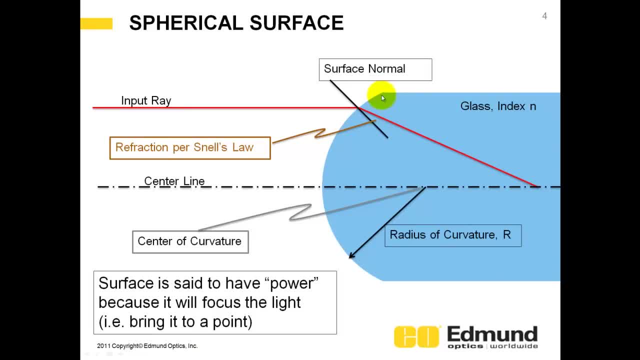 just discuss a simple spherical surface. So here we've got a piece of glass made of, and it's polished on the end of it, a spherical surface. So we have an input ray coming in. It's parallel to this center line which goes through the center of curvature, This surface. 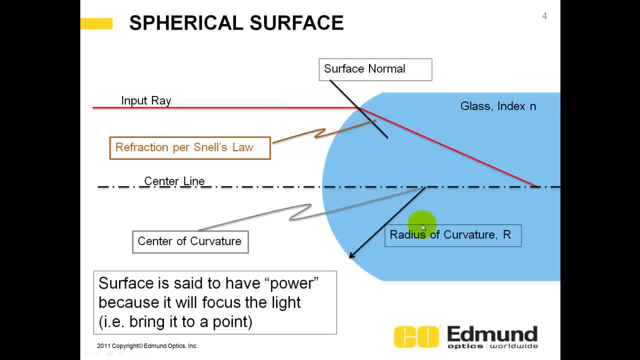 has a radius of curvature here, r, and we're not going to do any calculations with it. I'm just showing you what typical variables are used when describing the physics or the phenomenology behind this. So an input ray comes in and it's going to have there's 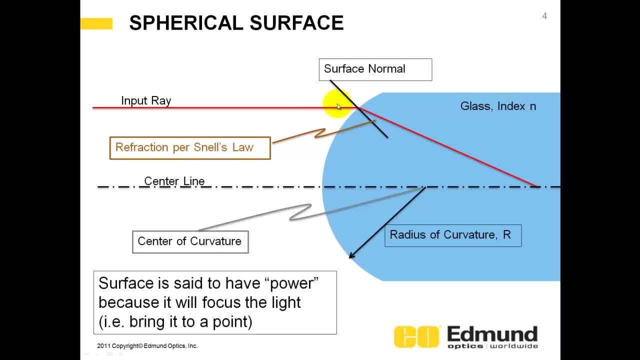 going to be a surface normal of this glass Right here And this light ray is going to refract per Snell's Law and this refraction angle here is going to follow again Snell's Law, assuming glass index of n. So this surface, 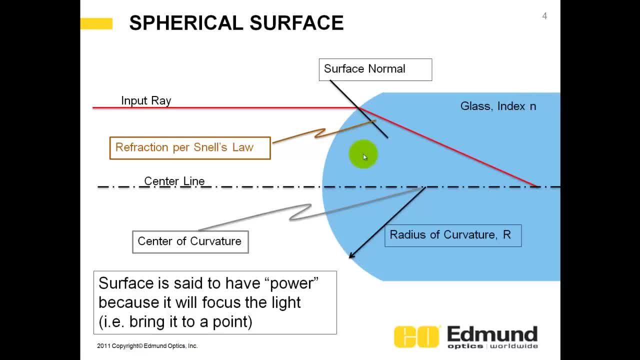 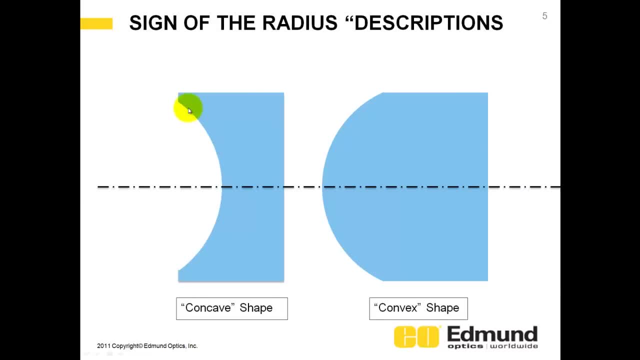 is said to have optical power because it focuses the light, In other words, it brings it to a point. Just for comparison, here is a surface with a concave shape and here is a surface with a convex shape. This will focus the light in the medium and this will 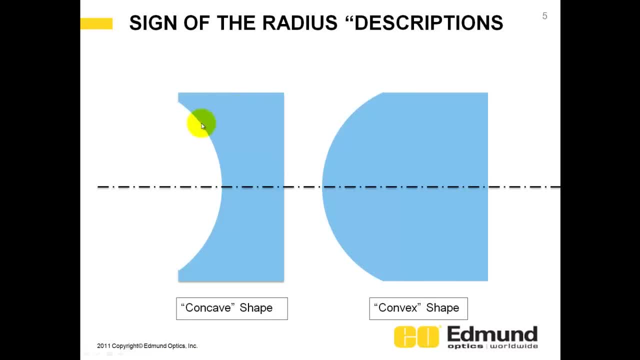 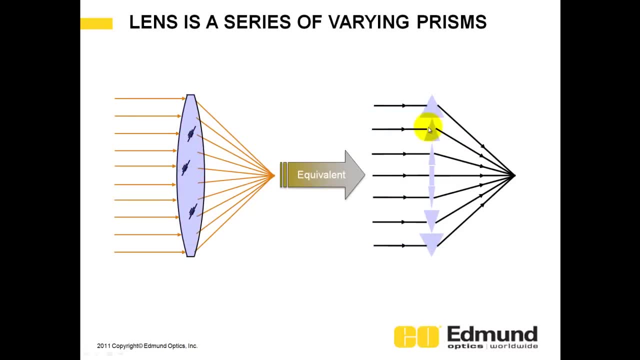 send the. the concave will send the light ray diverging. We'll talk about this a little later. Recall from last time that we started talking about prisms and how prisms bend light. So in this case we showed an equivalent model of what a lens is. So if you take a series, 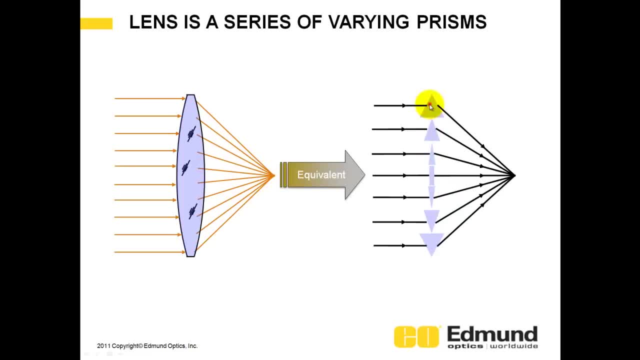 of prisms whose angle or the angle of the prism is equal to the angle of the lens, and its deflection or deviation increases with increasing aperture. you're going to bring the light to a focus, And that's exactly what a lens is doing. You've got a plain parallel. 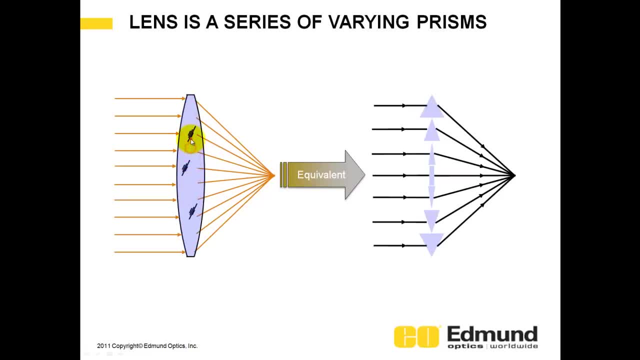 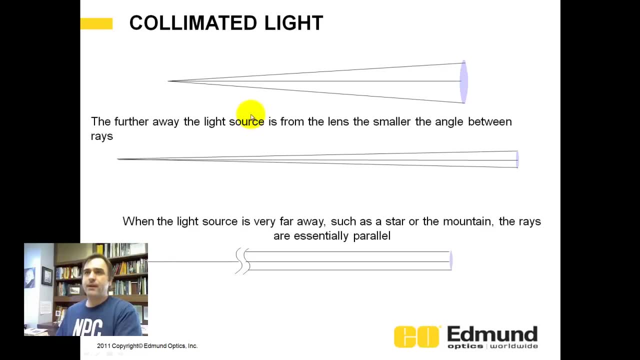 window right here in the center, and as you go out towards the end of the lens, you're getting a prism with a larger apex angle. I want to comment, I want to talk about collimated light. Recall that the wave front is based on the distance the wave is from the center. 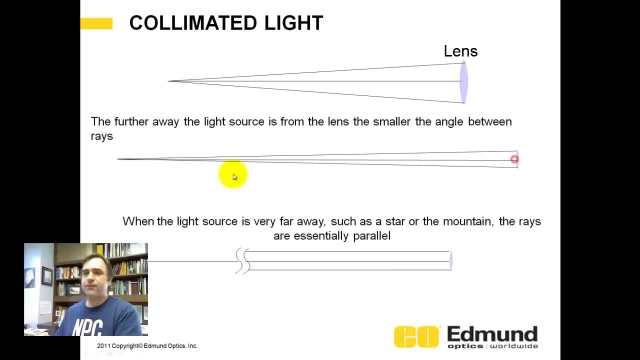 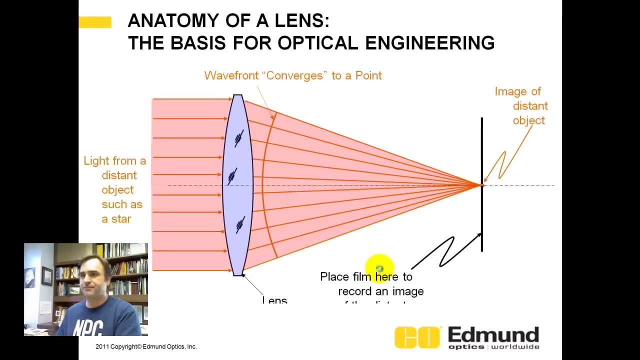 the point source. So as you get further and further away, your wavefront gets flatter and flatter. So if you're infinitely far away here, you're going to get a plane wave. And these rays here are all parallel, also called collimation or collimated light. Here's the 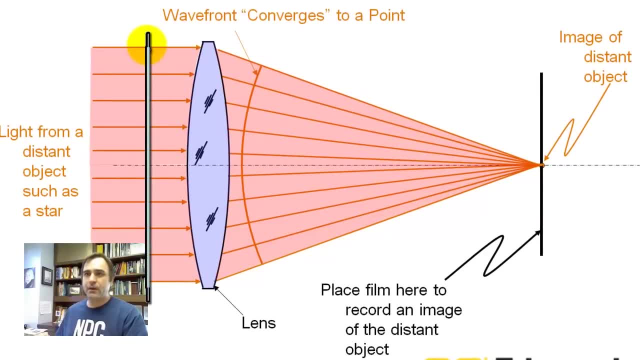 anatomy of a lens, of a basic lens. So here we have our plane wavefront here, collimated rays coming in. It's going to hit this lens, It's all going to bring it to the focus or the focal point. here This wavefront is converging, in other words coming to a point source. 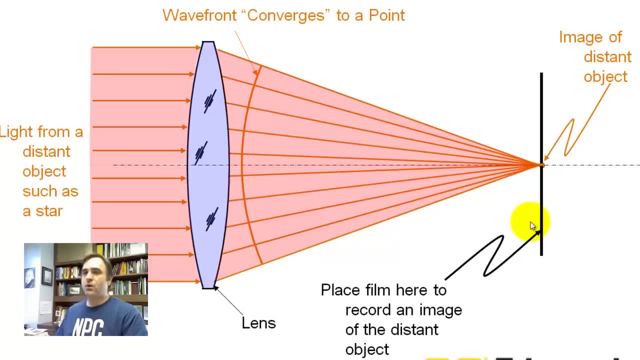 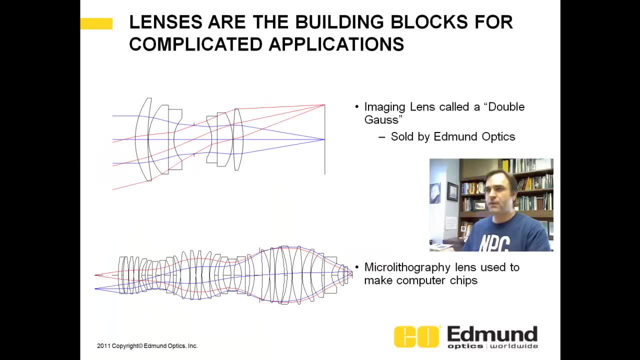 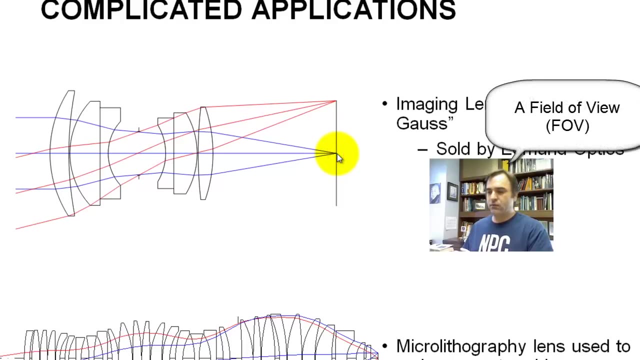 And this is your wavefront, after the lens. So if you want a camera, you put your film or your detector plane here and you're going to image that star. Now, you're not usually imaging a single point. You like to image a large area, a scene, several stars, the 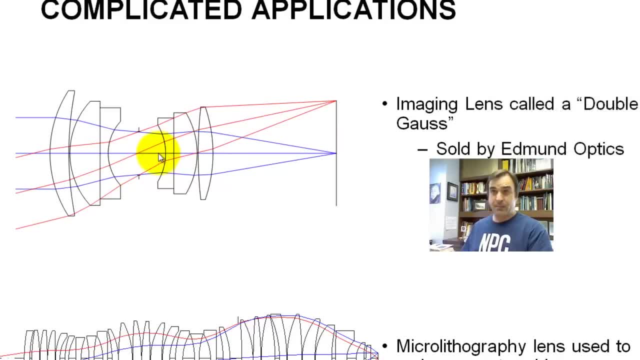 countryside, Whatever. So this top ray. here's some example of a more complicated lens assembly. This is called a double gauss. The blue rays are on axis forming this point, The red rays- so this might be looking at your kid, The red rays might be you know, the tree in the 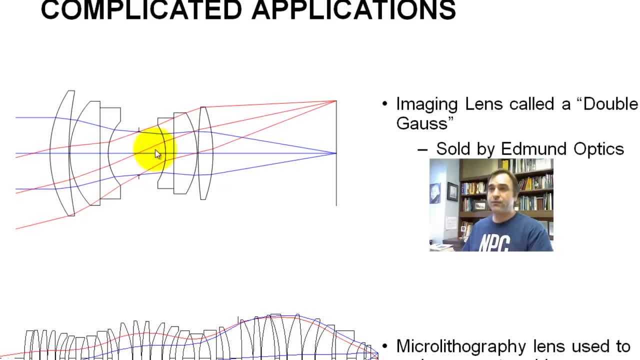 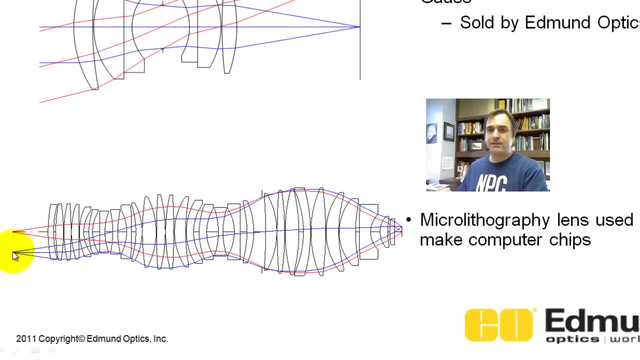 background. These red rays are coming off axis at a different field point and they're forming an image here. So this shows you you roughly need for a kind of a simple camera lens. you need six lenses carefully arranged, As opposed to a micro lithography lens. this is used. you put a photo mask here of what. 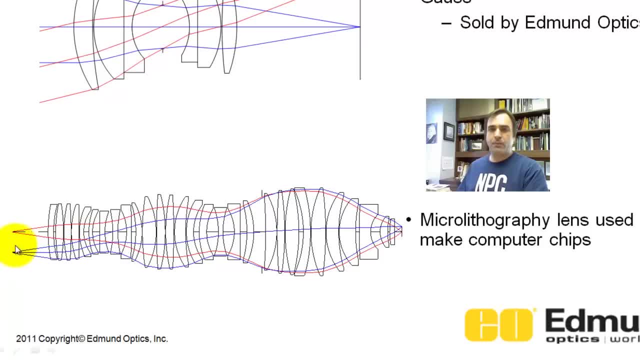 your, your electronic chip or computer processor is here and they use UV light back here to process and shrink down to make a smaller computer chip here. There's a lot of elements here because you it's hard to solve color, You've only got a few optical materials to. 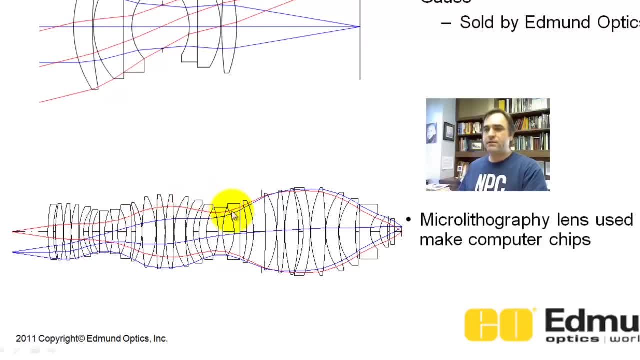 work with You're. these lenses and beams are changed. You can't see them, You can't control them. These beams are changing diameters to balance distortion- We'll get into distortion later. but an imaging system can be as simple as a lens or as complicated as you make it. 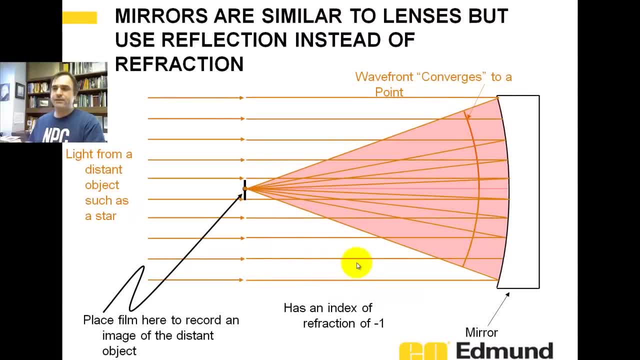 The analogy to a lens is a mirror and it's a single surface. It does the same thing: It's going to create a wavefront that converges to a single point And again it bounces back on itself. So a lens is continuous from left to right, whereas a mirror is going to go. 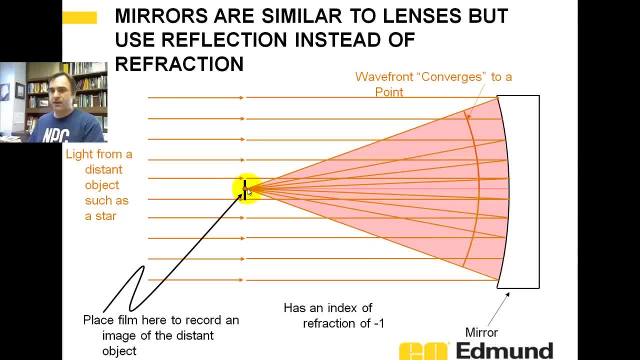 from left back and right. So here's where we're going to do a single mirror. This is to left back in on itself and for sake of when we get into equations. this mirror has an index of refraction of minus one, and want to just highlight that. you know the Hubble Space. 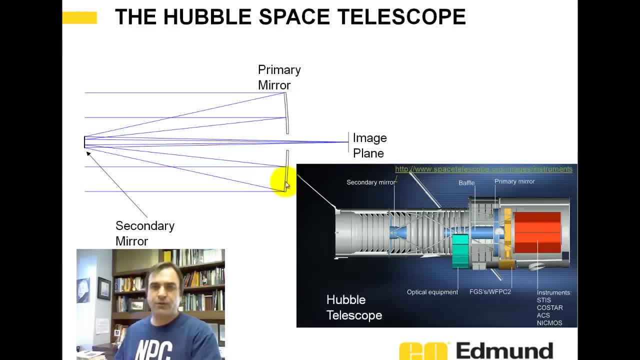 Telescope that everyone's aware of, that's, you know, orbiting the earth. that's done some great astronomy over the last decade or so. it's a caster grain. you've got a primary mirror here and a secondary mirror here in an image plane so you can see in the diagram. here's the primary, here's the. 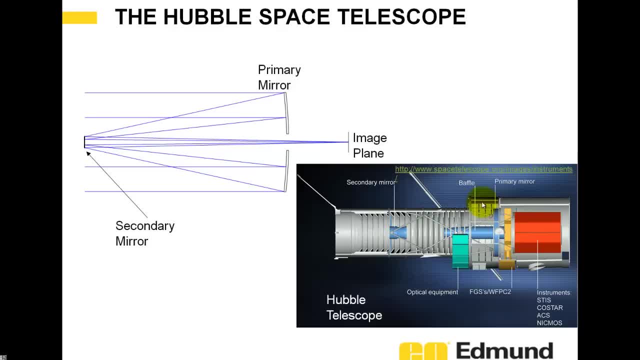 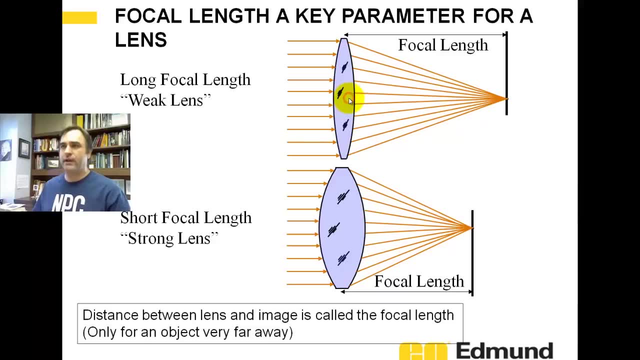 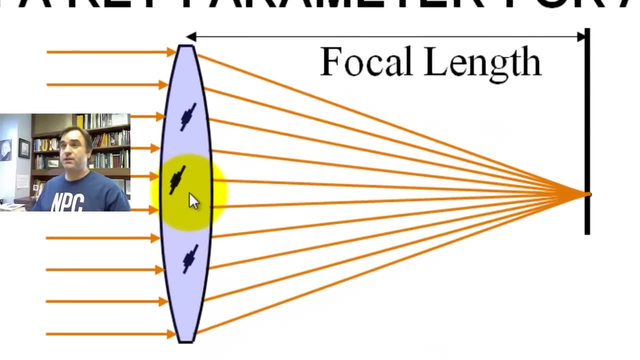 secondary, and here's all your instrumentation packages. let's talk about focal length. there's all kinds of lenses. let's compare a long focal length lens, which is on the top, to a short focal length lens. so what is focal length? focal length is essentially distance from the lens to where. 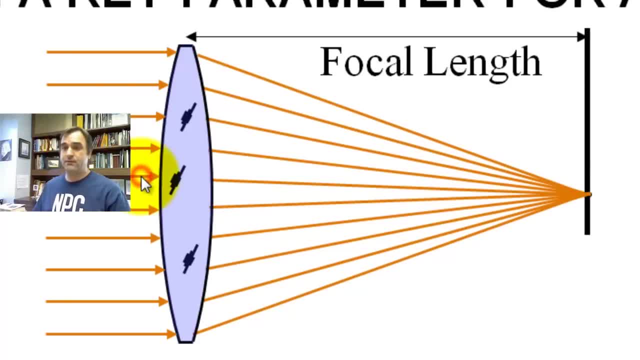 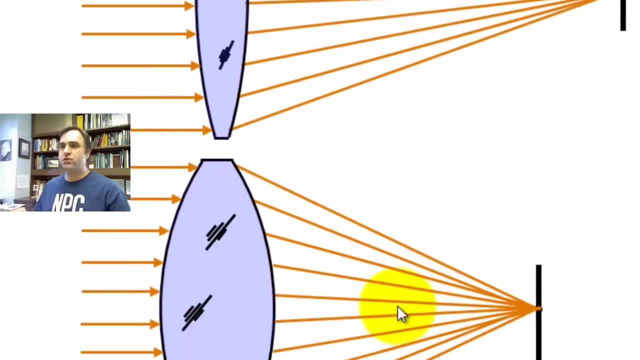 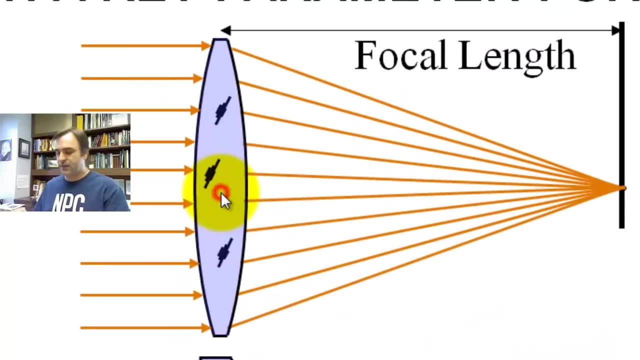 it focuses for collimated light. so the focal length: this is the focal length only when your light is infinitely far away. this is a long focal length, this is a shorter focal length. now notice, you have to curve your lens more, so we kind of say this is a strong lens, this is a weak lens. there are quantitative terms to describe a. 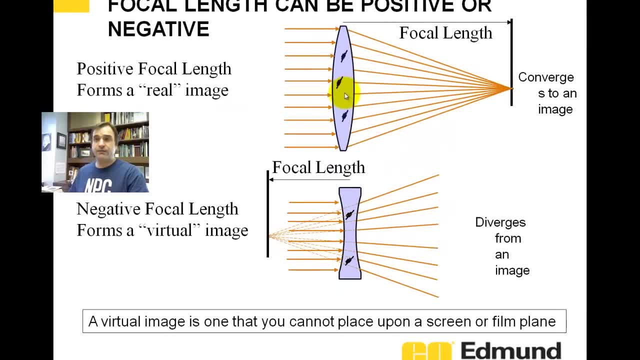 lens focal length can be positive or negative. this top one shows a positive focal length. this forms what we call a real image, because if you had a point source, a star coming through a lens, you could stick a piece of paper right here and you'll see a little dot form. there you're mapping. 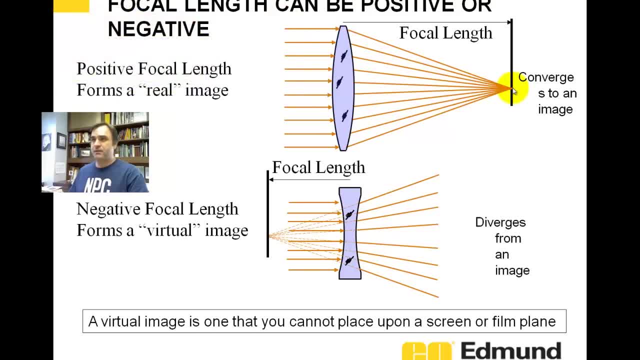 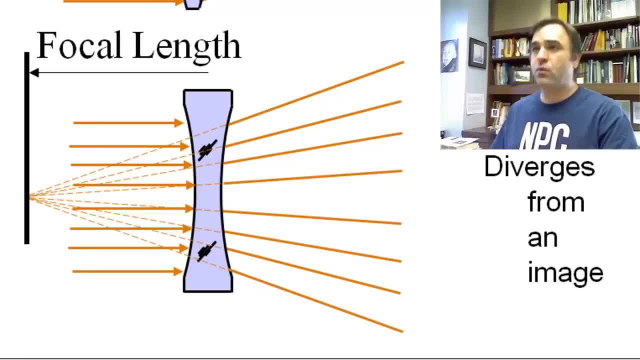 object space to image space. here, as opposed to a negative focal length, light's going to come in and it's going to diverge. so here we're converging to a point, here we're diverging from a point and we're diverging from a point that's back inside the lens. we call this. so this, this rate comes out, if you. 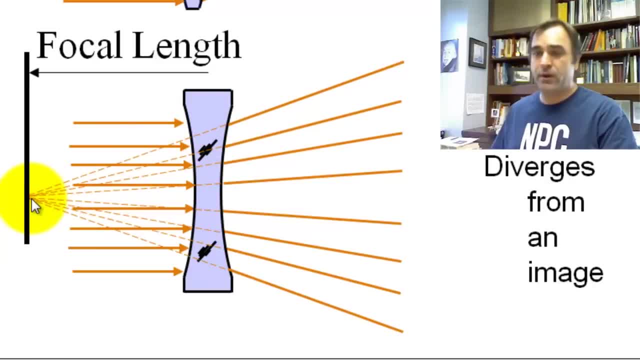 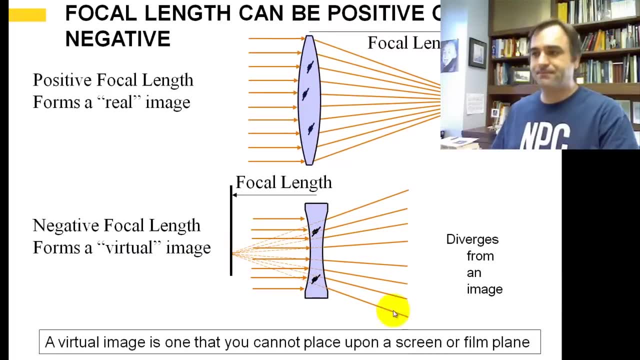 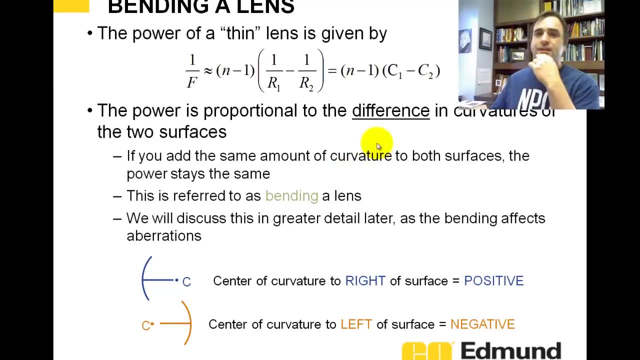 project it backнал where it originated. there's a focal point here, But it's called a virtual image because you physically can't get a piece of paper there to image that point. So let's talk about bending of a lens, And to do that I need to discuss the equations. 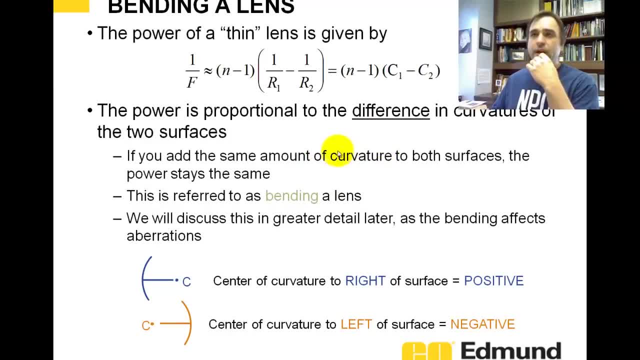 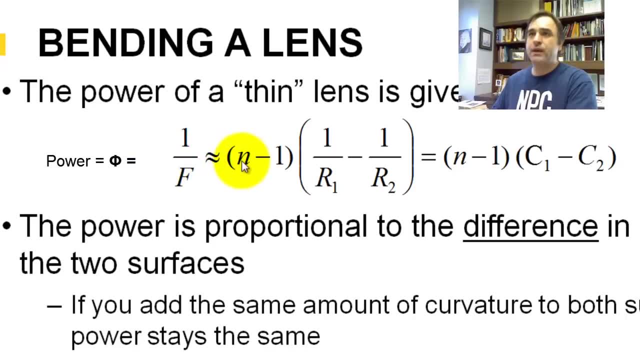 for a focal length of the lens. So a focal length or the inverse of the focal length is also called power. I should put a power term here. It's proportional to the index minus one times the difference between the curvatures And a curvature is one over the. 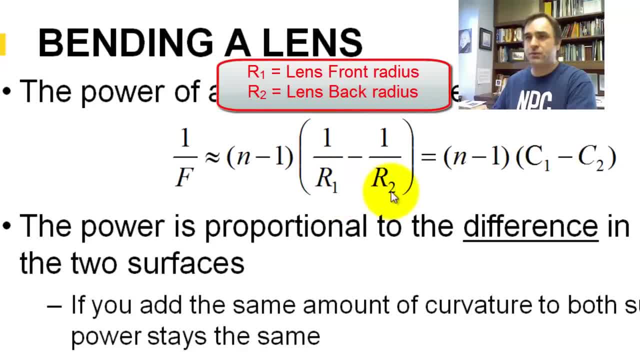 radius. So R sub one is the front, R sub two is the back. If we add a small amount to this curvature and the same amount here, we do not change the focal length. That's called bending, And we'll get into this in a little bit more detail, So you can have a certain 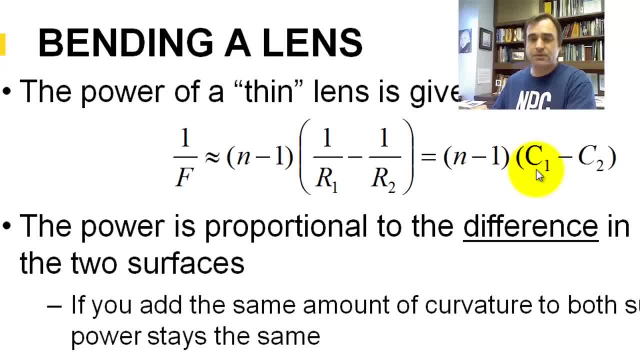 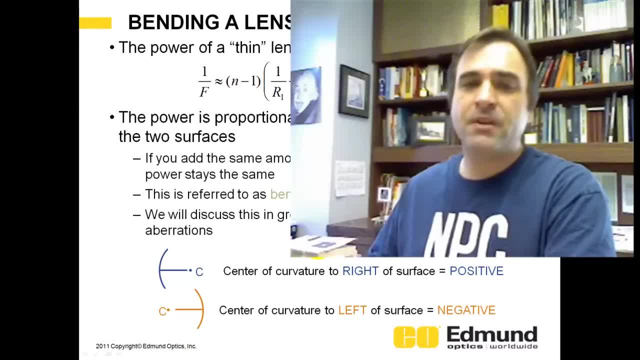 focal length lens that has all sorts of shapes and it's all got the same focal length And it's all got the same focal length, And it's all got the same focal length. I want to talk about sign convention a little bit. You've got to be very careful with sign. 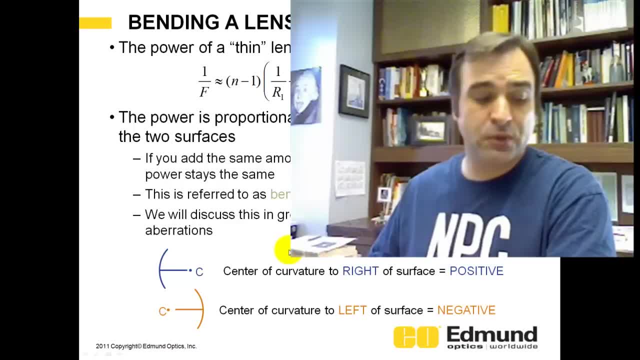 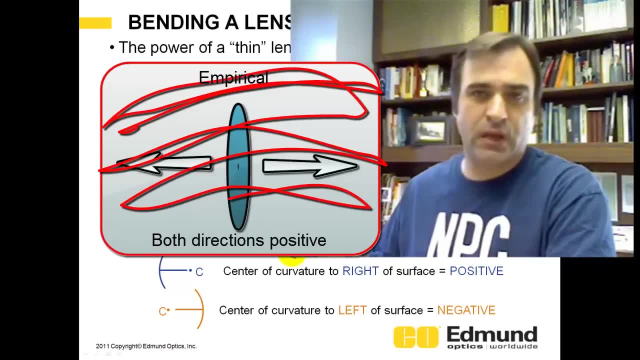 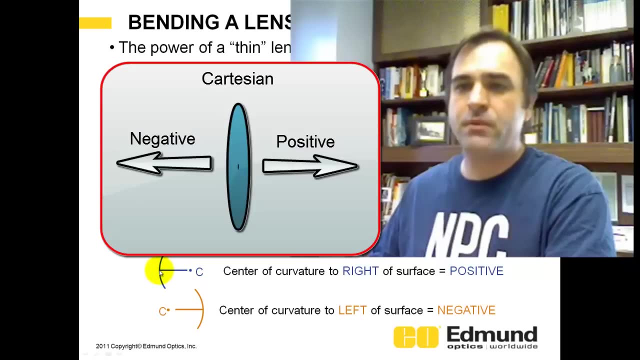 convention And some people use one. Some people use an empirical sign convention where distances to the right and left are both positive. Right and left of the lens are both positive. We're going to use the Cartesian coordinate system where distances from the surface to 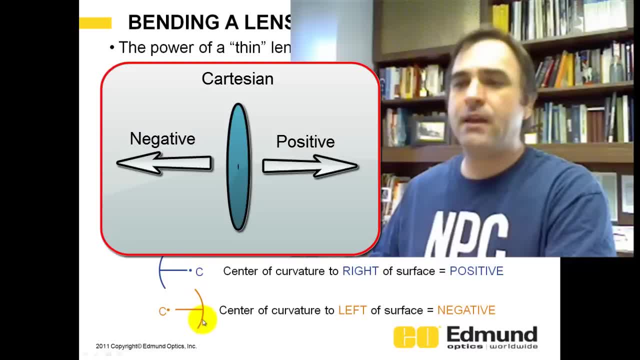 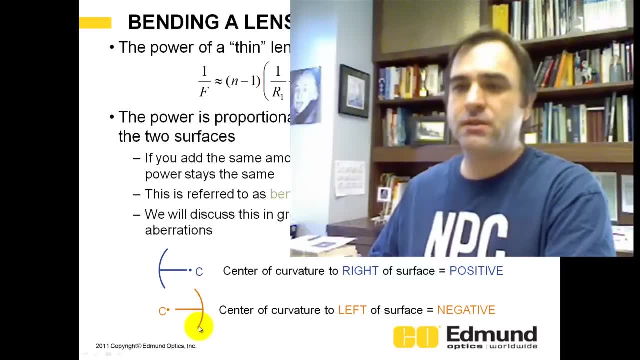 the right are referred to as positive And things measured to the left are negative. So, for instance, a concave curvature is going to be. let's say there's glass right here. this is concave. This is going to be a negative radius of curvature If we've got glass. 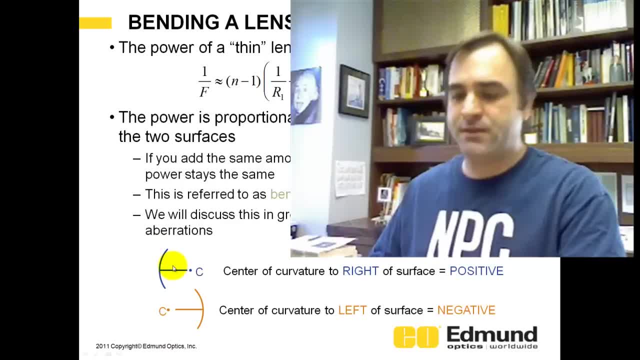 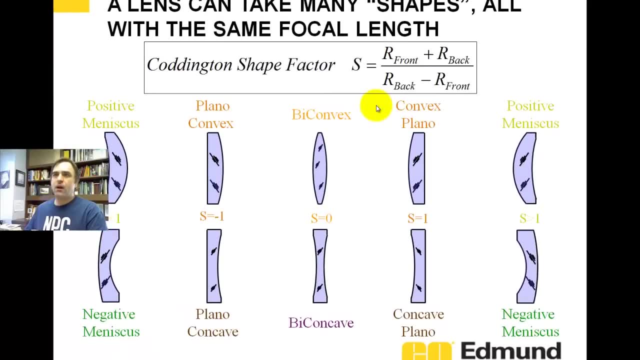 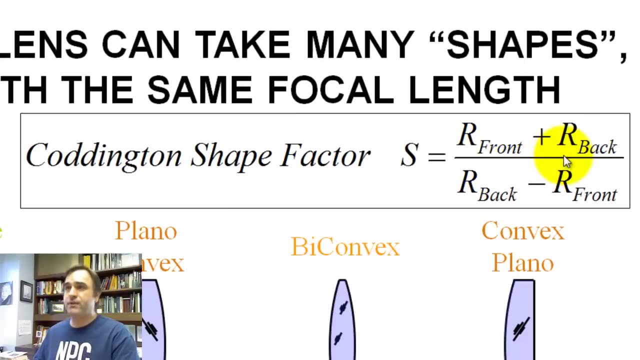 here and this is convex. this is a positive radius of curvature, So here's bending, Also called Coddington shape factor. So the shape factor is the sum of the radii divided by the difference. And notice the difference. you put the back radius minus the front. 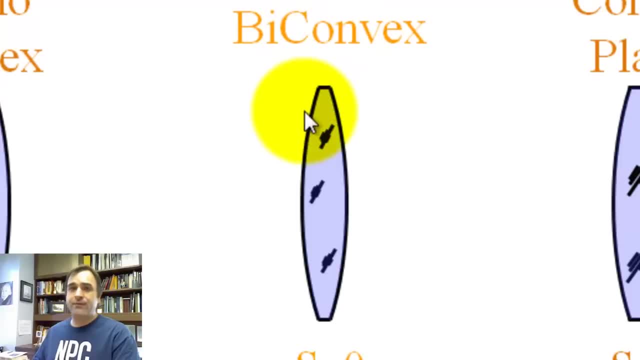 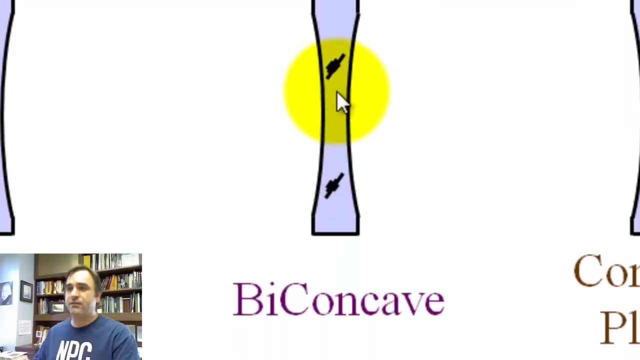 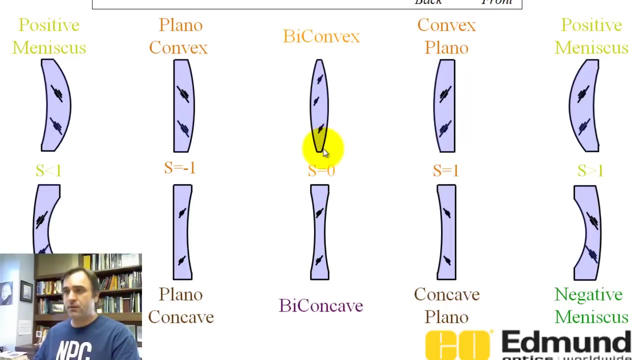 radius. So for lenses that have an equal radius to the front and back, here's a biconvex positive lens. This is a biconcave negative lens. Your shape factor is zero. As you increase, you're essentially bending. You go from, you know, bi to a convex plano or a concave plano out to a meniscus.